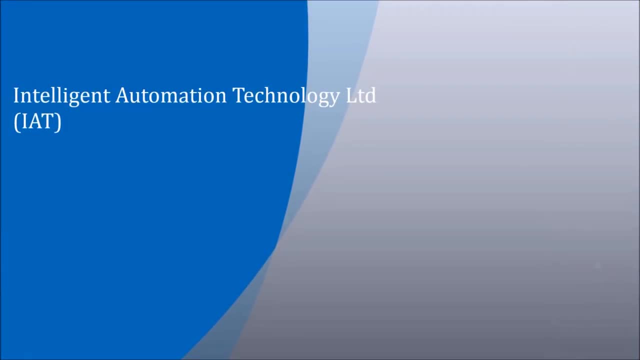 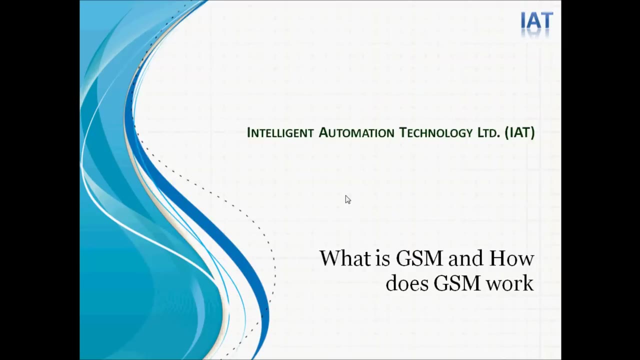 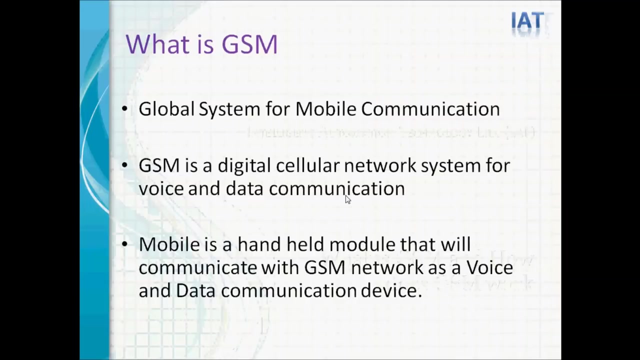 hello everybody. today I will try to give you a brief description on GSM. what is GSM and how does it work? what is GSM? GSM stands for global system for mobile communication. This is a cellular network system for voice and data communication. Mobile equipment- mobile, which is a handheld device. 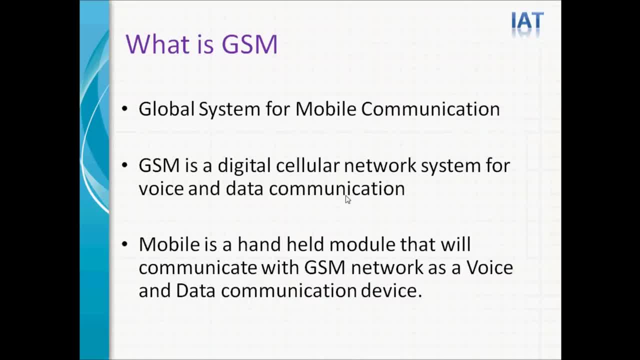 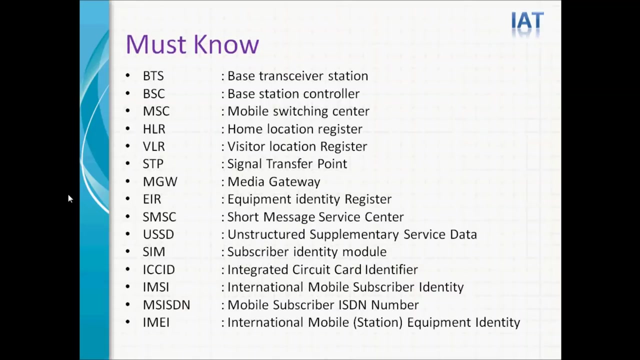 will communicate with GSM network as a voice and data communication device. currently, data communication device is separately available. before having the description, you must know about this short tab that we will use in this video. first the presentation: BTS means for Base Transfer Station, VSC Base Station. 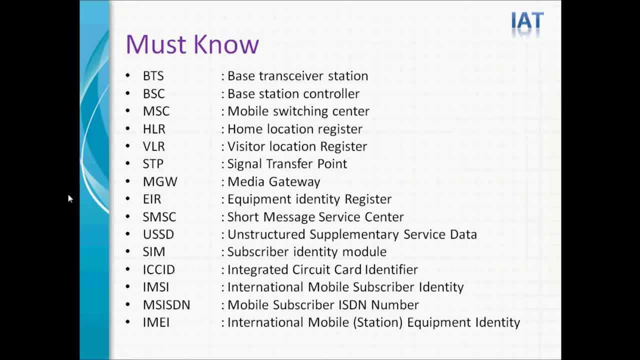 Controller: MSC Mobile Switching Center. HLR Home Location Register. VLR Visitor Location Register. STP Signal Transfer Point, MGW Media Gateway, EIR Equipment Identity Register. SMSC Short Message Service Center, VSST and Structured Supplementary Service Center. 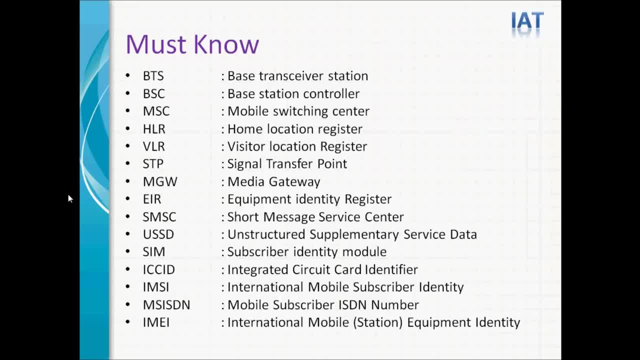 Short Message Service Center VSST and a structured supplementary service center. short message service center vsd and a structured supplementary service center. and a structured supplementary service center and a structured supplementary service center. Service Data SIM Subscriber Identity Module. ICCID- Integrated Circuit Data Identifier. 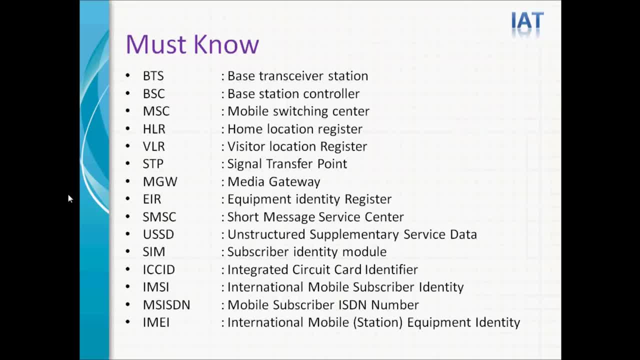 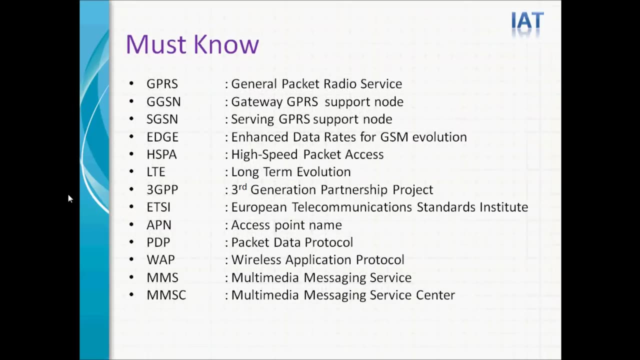 IMSI International Mobile Subscriber Identity. MSISDN Mobile Subscriber IDN Number. IMEI International Mobile Equipment Identity. GPRS General Packet Radio Service. GGSN Gateway GPRS Support. Note. SGSN Serving GPRS Support. Note: IS Enhanced Data Rates for GSM Evolution. 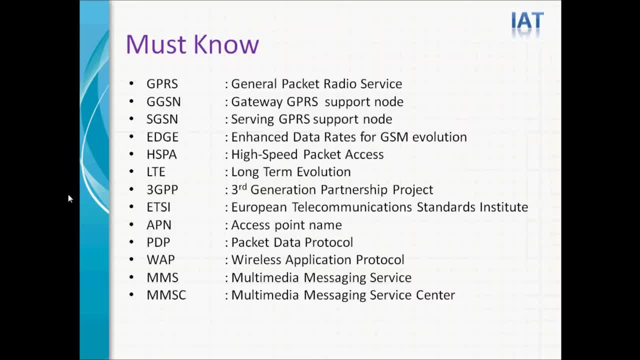 HSPA High Speed Packet Access LTE Long Term Evolution, 3GPP Third Generation Partnership Project, HC- European Telecommunications Standards Institute. APN Access Point Name: PDP Packet Data Protocol, WAP, Wireless Application Protocol, MMS, Multimedia Messaging. 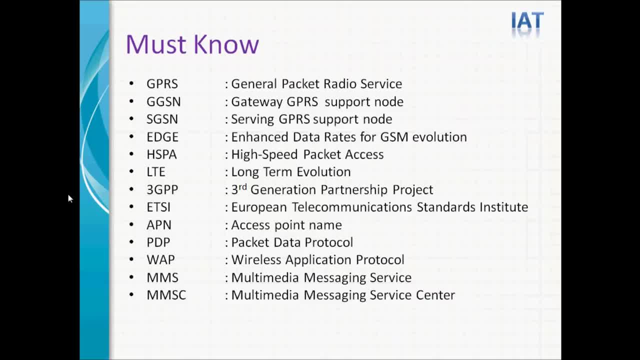 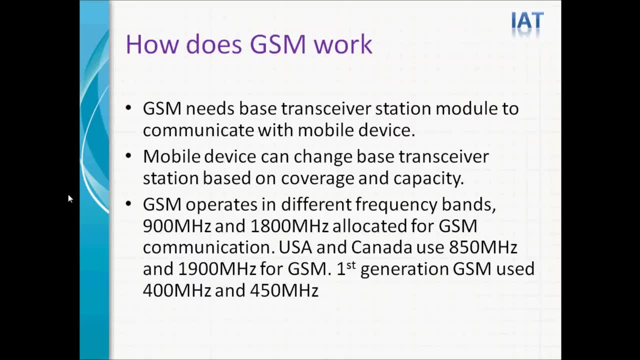 Service, MMSC Multimedia Messaging Service Center. How does GSM network work? How does GSM work? GSM needs Base Transceiver Station Module to communicate with mobile device. Mobile device can change Base Transceiver Station based on power range and capacity. GSM operates in different frequency bands- 900 MHz and 1800 MHz, allocated for GSM communication. 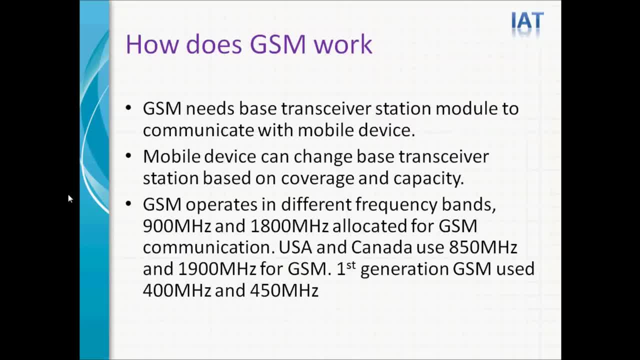 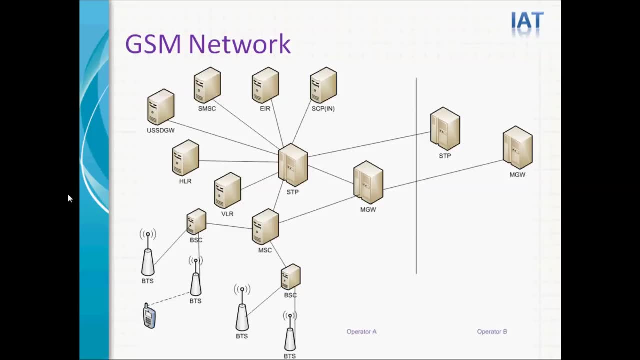 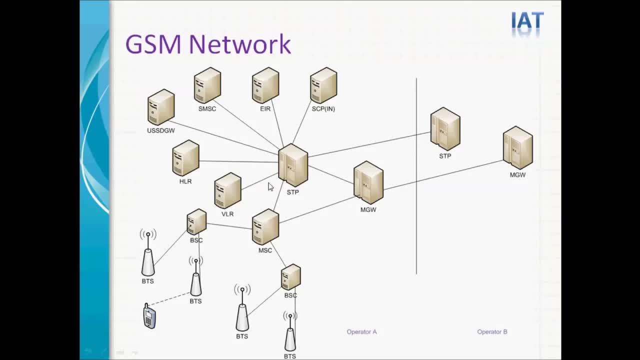 This is the basic architecture of GSM network. STP is the centre for GSM network. In case if the network don't have an STP, MSE is the centre of this network. Here STP is the signal transfer point. All other nodes are connected with this STP for the signal communication. 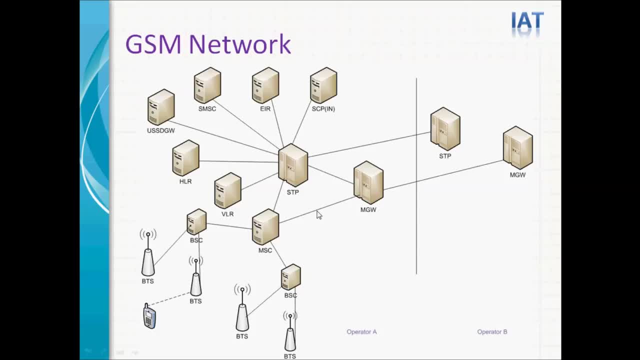 media gateway. this is for the voice gateway, for this to STP and media gateway connected with the external network. for example, if you have more than one operator, the inter operator communication for the signaling can be done between the STP to STP and voice communication. the trunk will be. 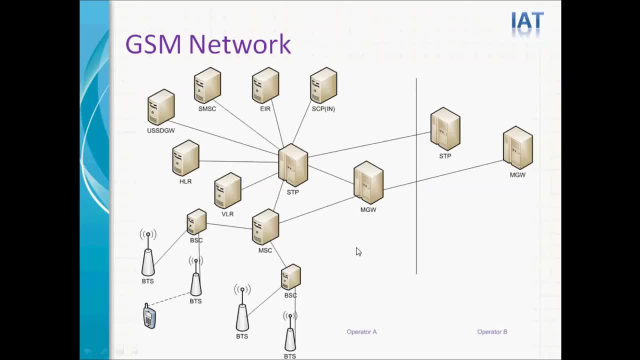 connected between media gateway. if the field level network is the VTS, all mobile devices communicate with this VTS. at the group of VTS connected with VSC and MSC can cover more than one VSC. in a network there can be more than one MSC and the other nodes are processing the signaling only, only the. 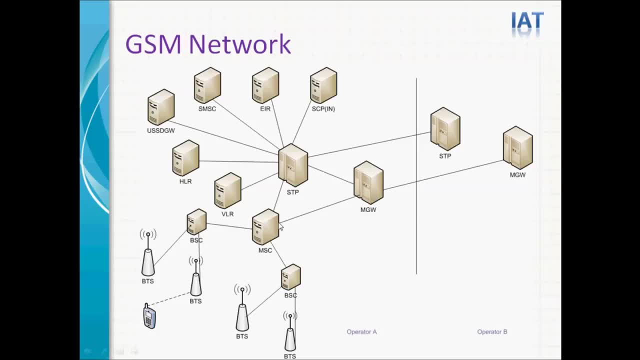 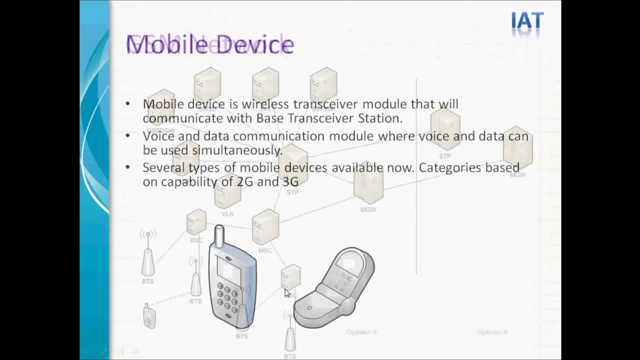 MSC and the media gateway. in the core part they are communicating for the voice. let's have a description for each item in the GSM network: mobile device: a while device is a wireless transceiver module that will support the facility and also adjust the signal consensus communicate with the VTS voice and data communication module. wire voice and data. 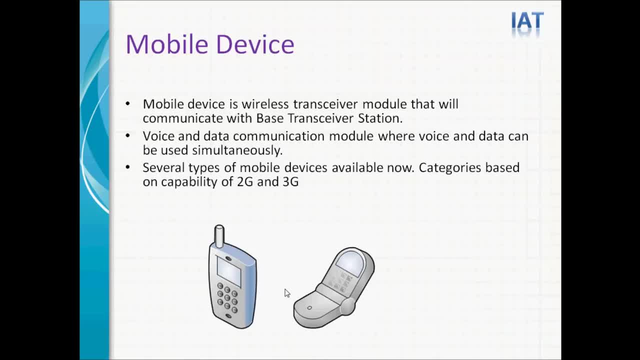 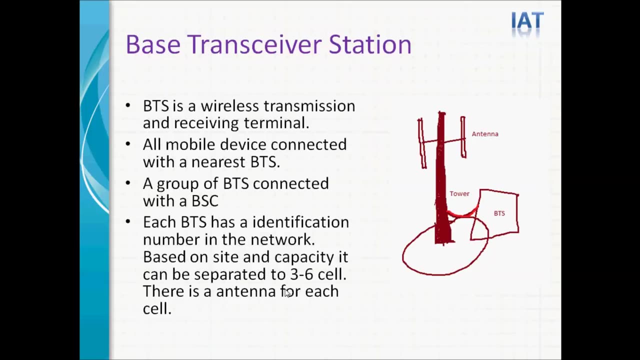 can be used simultaneously. currently, several types of mobile devices available in the market based on the 2G and 3G base transceiver station. VTS is a wireless transmission and receiving terminal. all mobile device connected with a nearest VTS. a group of VTS will be connected with a VSC. each VTS has 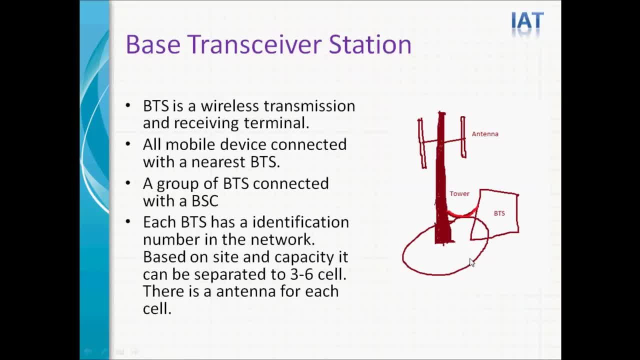 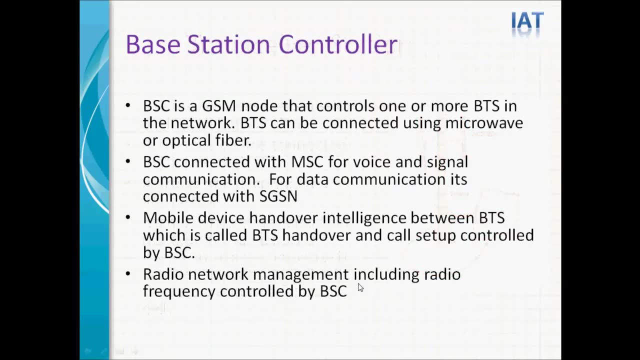 identification number in the network. based on site and capacity. it can be separated to two to six cell for every cell. there should be an antenna that will cover this cell base station controller. VSC is a GSM note that controls one or more bts in the network. bts can be connected using microwave or optical fiber. 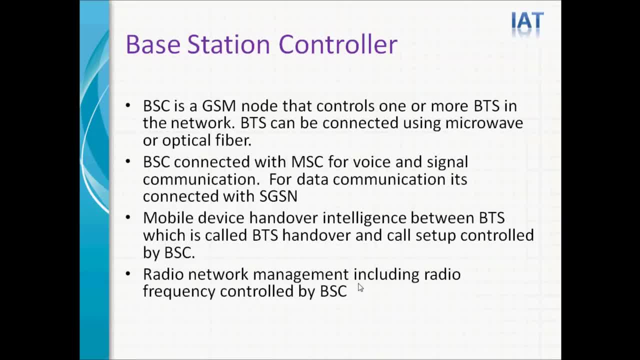 bsc connected to the msc for voice and signal communication. for data communication it's connected with sgsm mobile device handover intelligence between bts, which is called vts handover and call setup control by bsc. radio network management, including radio frequency controlled by bsc. 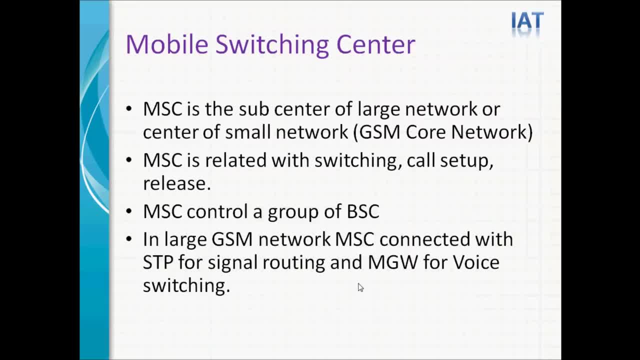 mobile switching center. msc is a sub center of large network or center of small network. ms is part of json core network message related with switching. call setup release. msc control a group of bsc in large gsm network. msc connected with sdp for signal routing and media gateway for voice switching. home location register: hlr. 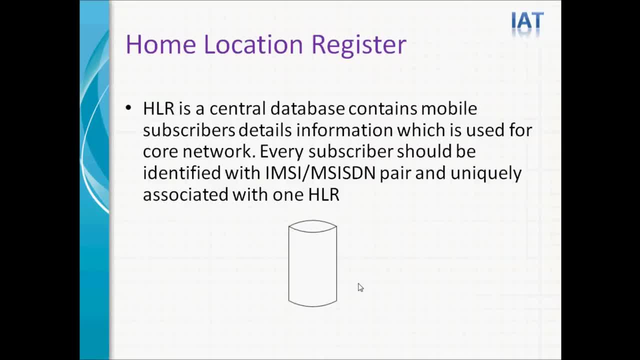 is a central database contains mobile subscribers detailed information which is used for poor network. every subscriber should be identified with img and msisdn pair and uniquely associated with one hlr. in a network, there can be more than one hlr based on the subscriber number prefix. 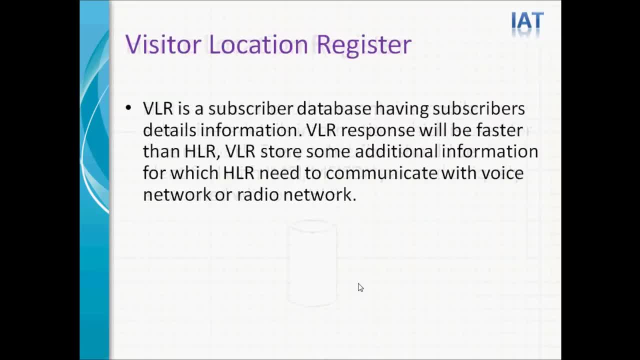 hlr can be separated visitor location register. vlr is a subscriber database having subscribers details, information, vlr response will be faster than hlr vlr. vlr stores some additional information for which hlr need to communicate with voice network or radio network. vlr will reduce the cost so that for call communication on the other part. 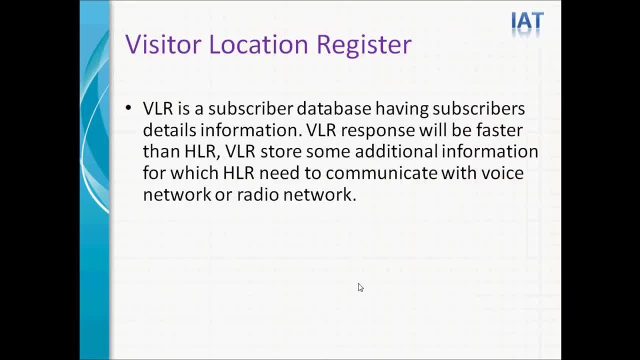 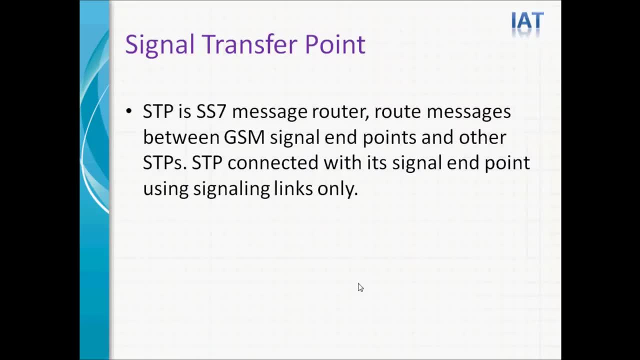 the other node don't need to communicate with hlr every time. they can communicate with vg vlr for getting the source neighbor information. signal transfer point stp is ss7 message router route messages between gsm signal endpoints and other stps. stp connected with the signal endpoint using signaling links only. 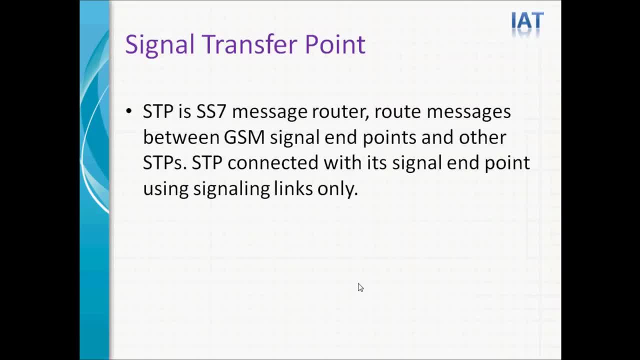 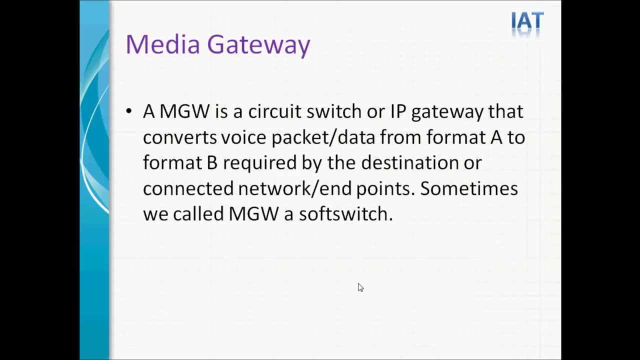 stp will not handle any voice related traffic or other voice related data. media gateway is a circuit switch or ip gateway that converts voice packet data from i2 format b required by the destination or connected network or endpoints. sometimes we call the media gateway as a soft switch. 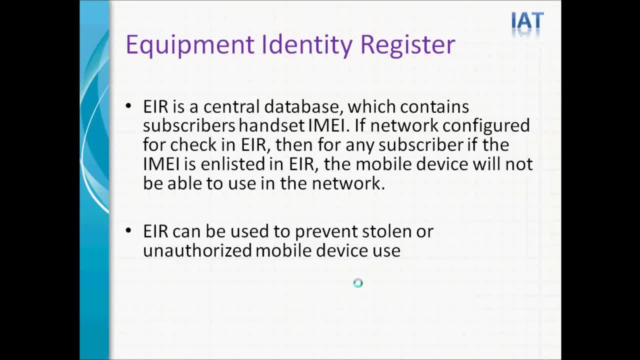 eir equipment identity register is a central database which contains subscribers handset imei. if network configured for check in eir, then for any subscriber if the imei is enlisted in iir, the mobile device will not be able to use in the network either. can be used to prevent stolen or unauthorized mobile device use. 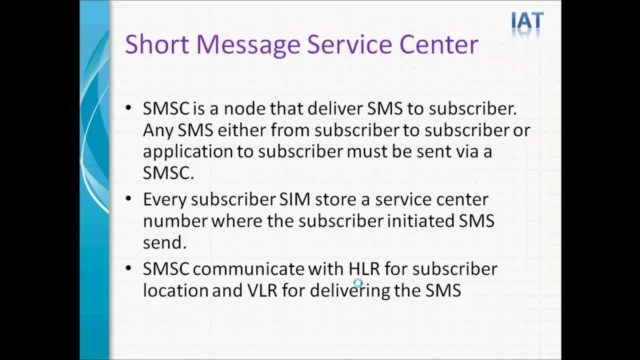 short message service center, smsc, is a node that deliver sms to subscriber. any sms, either from subscriber to subscriber or application to subscriber, must be sent by a smsc. every subscriber see store a service center number where the subscriber initiated sms. send sms, communicate with hlr for subscriber location and vlr for delivering the sms. 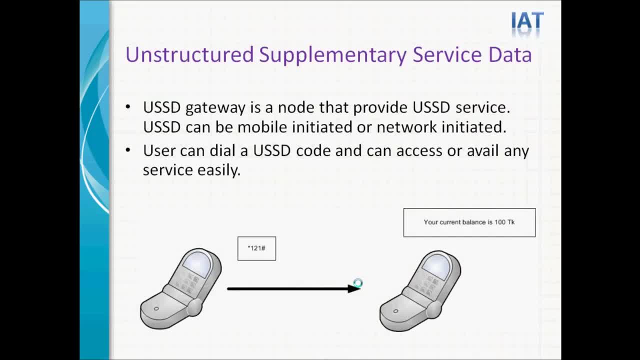 ussd, an unstructured supplementary service data. to have a ushd service network must have ushd gateway. ussd gateway is a node that provides ussd service. ussd can be mobile initiated or network initiated. user can dial ussd code and can access or avail any service easily. 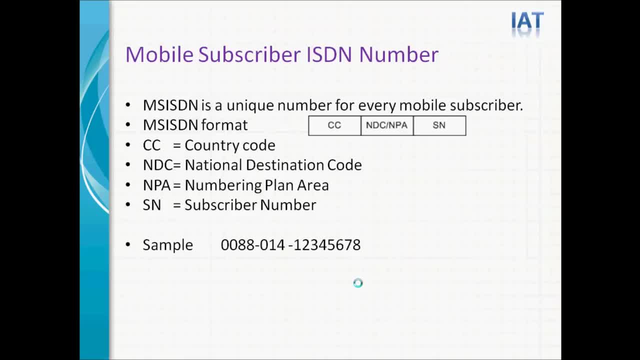 mobile subscriber isdn number. msisdn is a unique number for every mobile subscriber. msisdn format have three field. cc is for country code. mdcnpa is a national destination code or number in plan area. sn is the subscriber number. the sample here: zero, zero, eight, eight is the country code for bangladesh. 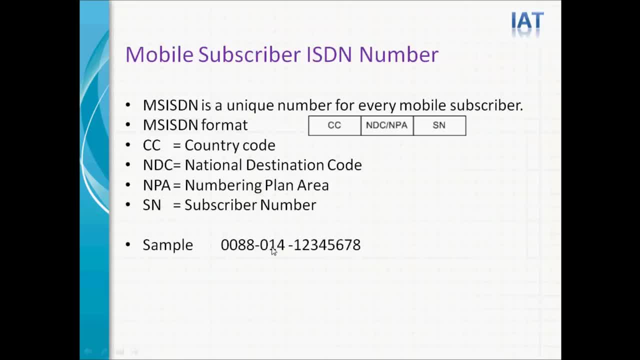 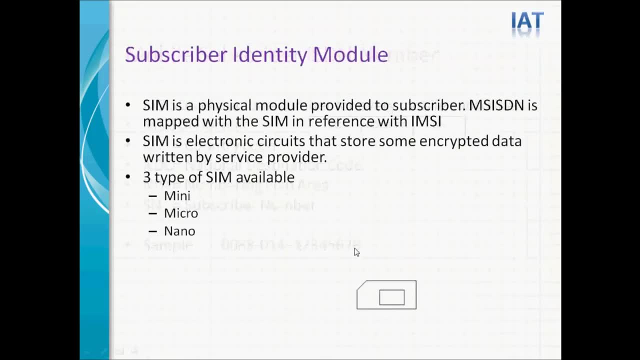 zero. one. four is the national destination code. this is the operator code and last eight digit is a serial number. subscriber identity module is a physical module. ещё one here, single number, is in tab one. we can see if we can output the speed. the ckd is the singer to be to make, always of ussd. it contains part from user code. 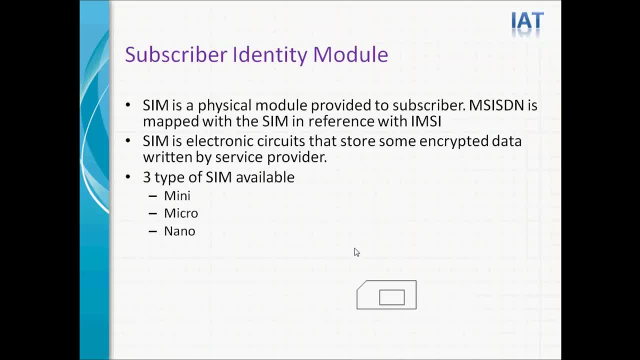 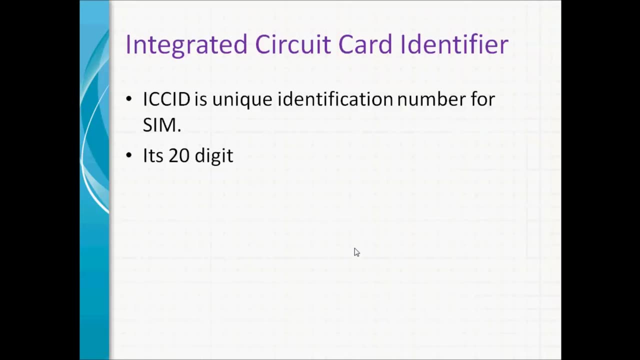 its doesn't add up to well. thats not what the user wn't to. let's girls, if they want it, will choose that. then select it. this is something that we are using. it will unwillingly tenho so using this 이걸 providerceica server. that's the way it is. 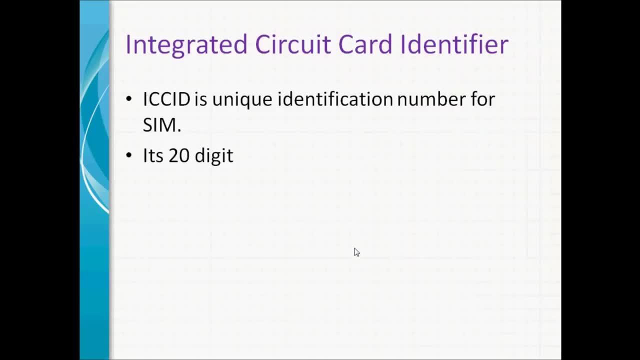 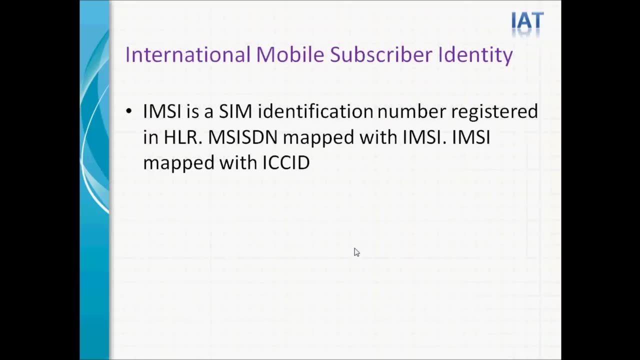 you can then set up a client and also the policy should be a set up as follow: by the server, a 20 digit number. IMZI- International Mobile Subscriber Identity. IMZI is a SIM Identification Number registered in HLR, MSIDN, mapped with IMZI. 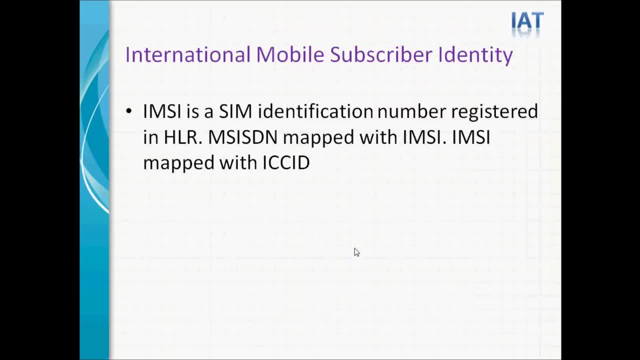 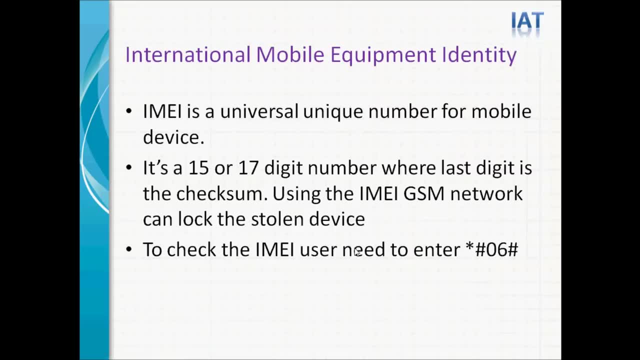 IMZI, mapped with ICCID International Mobile Equipment Identity, is a Universal Unit Number for Mobile Device. It's a 15 or 17 digit number where last digit is the checksum. Using the IMZI GSM network can lock the stolen device. 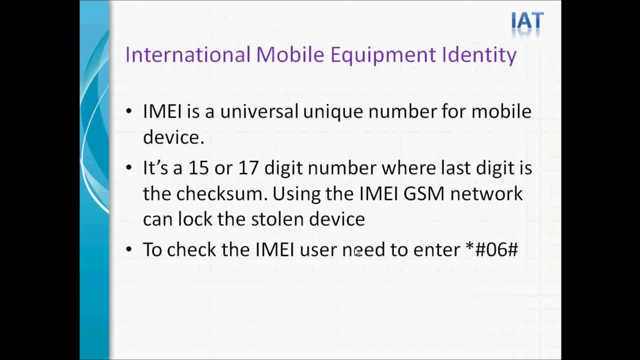 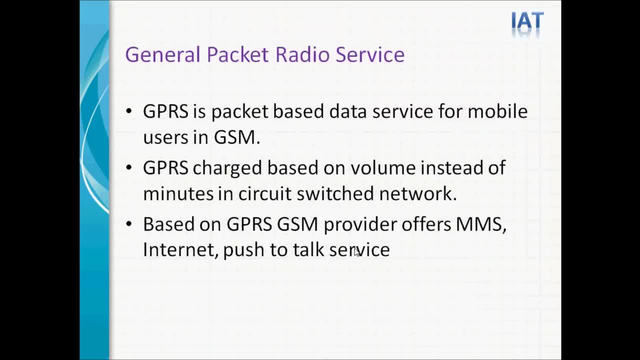 To check the IMZI, user need to enter star 06H and on the display he will get the IMZI of his device. General Packet Radio Service, GPRS, is packet-based data service for mobile users in GSM GPRS, charged based on volume instead of minutes in circuit switch network. 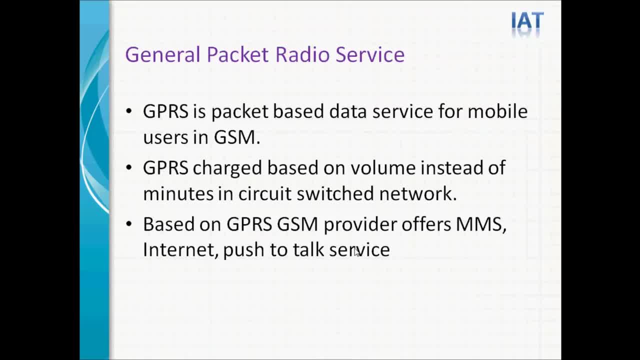 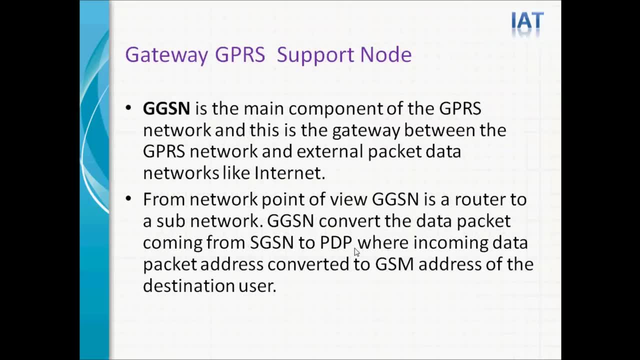 Based on GPRS GSM provider offers MMS, Internet push-to-talk and other services. GGSL is a Gateway GPRS support node which is the main component of the GPRS network And this is the gateway between the GPRS network and GTSL. 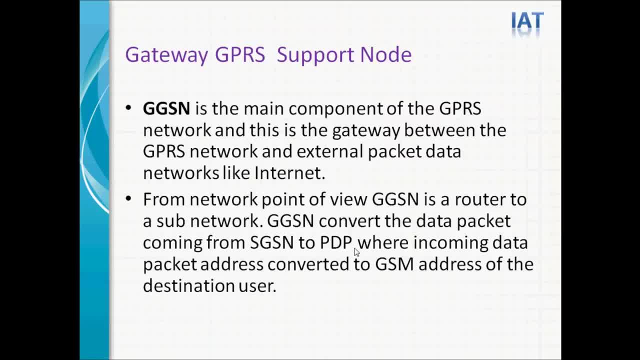 GTSL is the gateway between the GPRS network and GTSL. GTSL is a gateway between the GPRS network and external packet data networks such as Internet. From network point of view, GGSN is a router To a sub network. GGSN convert the data packet coming from GGSN to PTP, while incoming data. 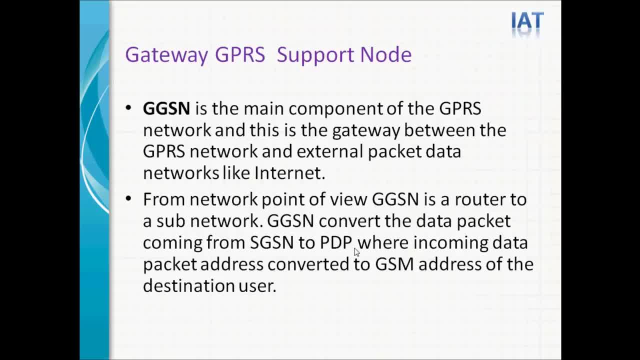 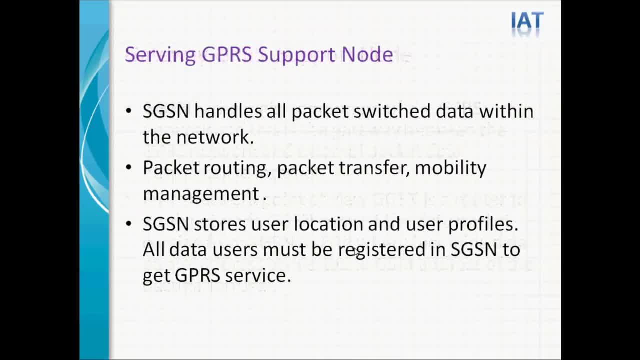 packet address converted to GSM address of the destination user. Here comes the mobile user Serving GPRS support node is the GSN. sgsn handles all packets with data within the network: packet routing, packet transfer, mobility management. sgsn stores user location and user profiles. all data users must be registered in. 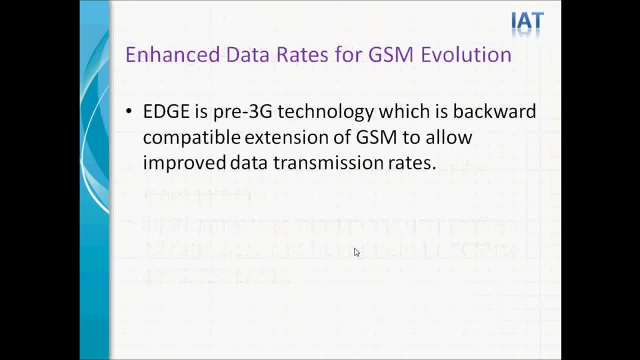 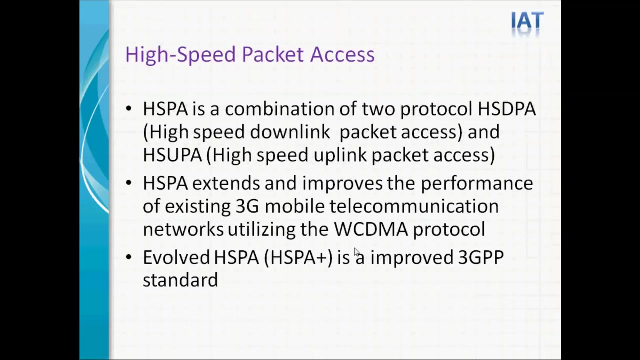 this gsm to get. gprs service is enhanced database for gsm. evolution s is a pre-3g technology which is backward compatible extension of gsm to allow improved data transmission rates. hspa- high speed packet access. hspa is a combination of two protocol: hsdpa- high speed. 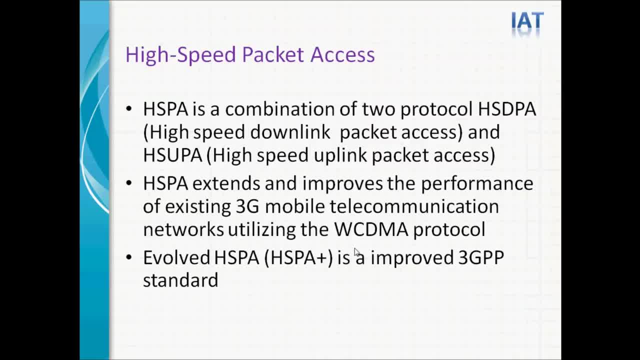 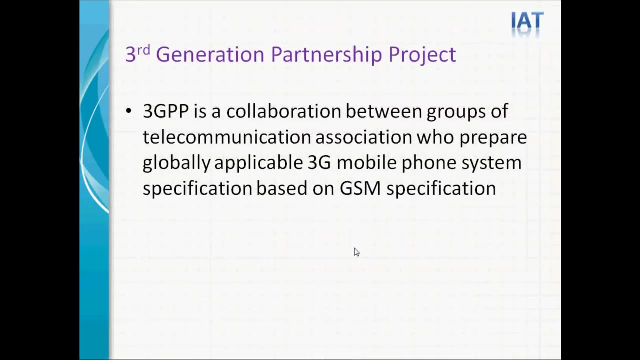 downlink packet access and hsu pa high speed uplink packet access. hspa extends and improves the performance of existing 3g mobile telecommunication network utilizing the wcdme protocol. evolved hspa. hspa plus is a improved 3g bp standard third generation partnership project 3g pb. 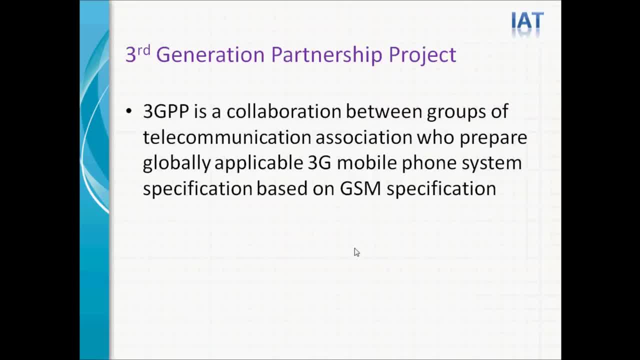 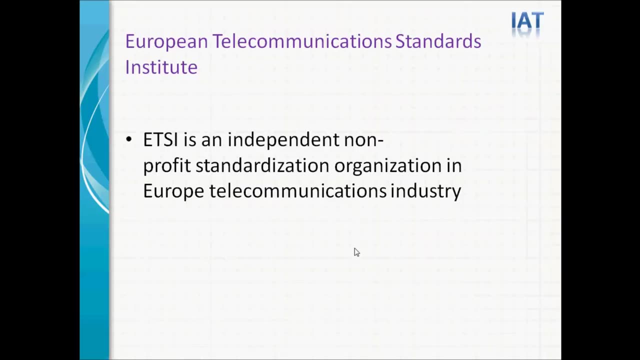 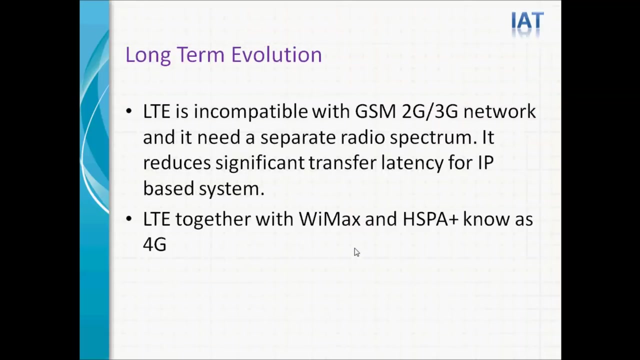 is a collaboration between groups of telecommunication association who prepare globally applicable 3g mobile phone system specification based on gsm specification. atc, european telecommunications standards institute is an independent, non-profit standard organization in europe. telecommunications industry. long-term evolution lte is an incompatible with gsm 2g 3g network and it needs a separate radio spectrum. it reduces significant transfer. 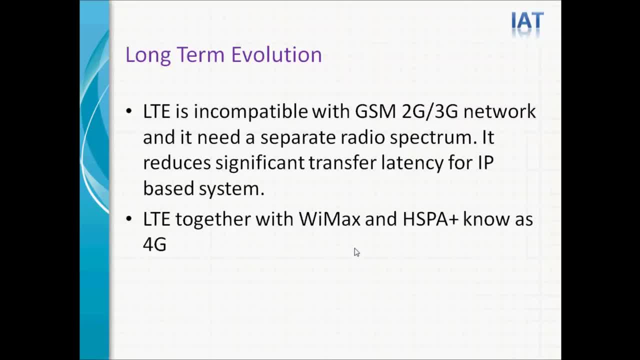 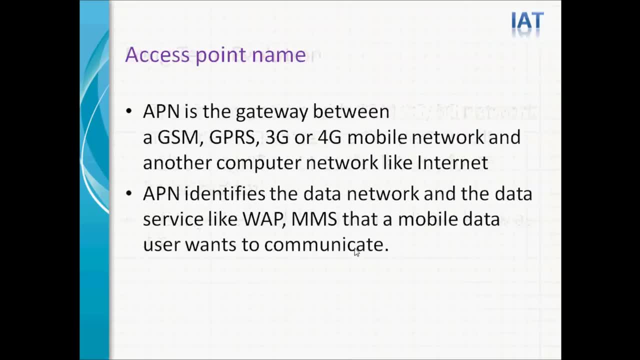 latency for ipv system lte. together with ymax and hsp and onus 4g access point name. apn is the gateway between a gsm, gprs, 3g or 4g mobile network and another computer network like internet. apn identifies the data network and the data service. 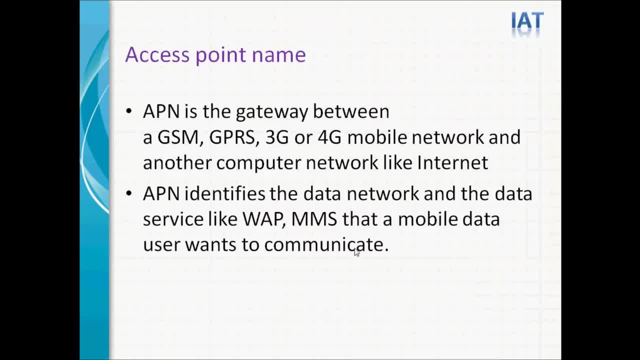 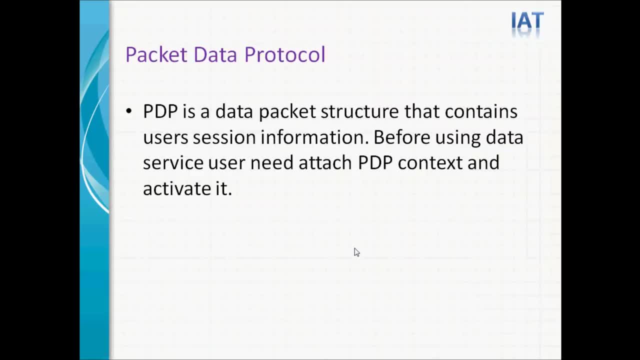 like wap mms that a mobile data user wants to communicate. pdp is packet data protocol is a data packet structure that contains user data that is not in the data package structure and that contains users session information. before using data service, user need attach pdp content. 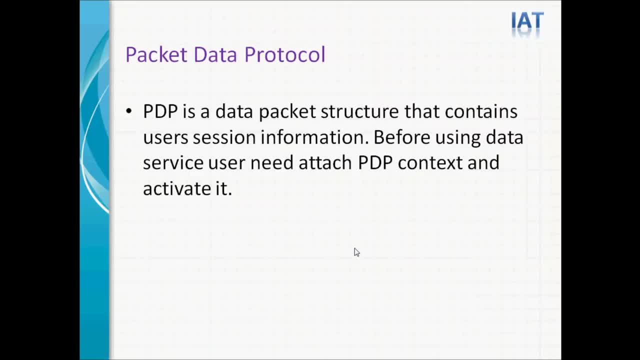 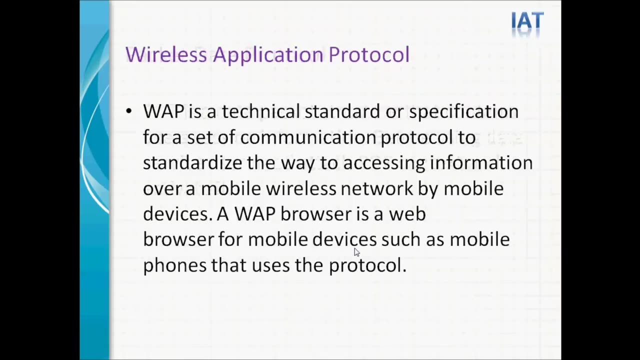 pdp packet data protocol. pdp is a data packet structure that contains user session information. before using data service, user need to attach pdp context and activate it. wireless application protocol is a technical standard or specification or a set of communication protocol to standardize the way to accessing information over a mobile wireless.